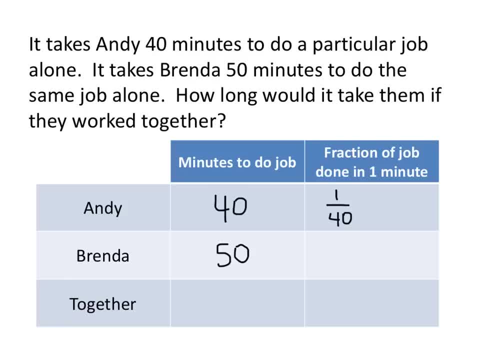 Similarly, Brenda takes 50 minutes to do the job, and so in each minute she gets one fiftieth of that job done. Now together, we don't know how much time it takes them to do the job, So we'll just call that t. 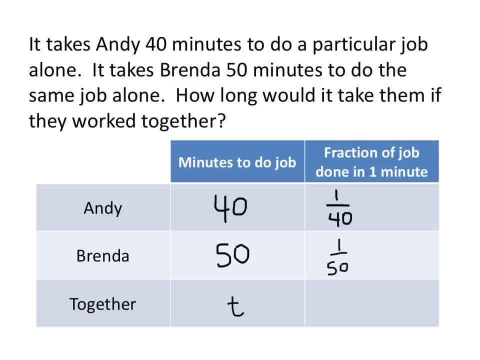 But what we do know again, thinking about what we talked about before, is that in one minute they will get one over t. That'll be the fraction of the job that they get done in each minute. But since they're working together, the amount of work that Andy gets done in one minute. 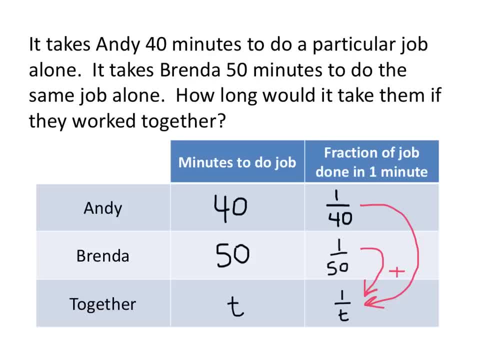 plus the amount of work that Brenda gets done in one minute. if we add those two amounts of work together, we'll get the amount of work that they get done together. So if we add one fortieth to one fiftieth, 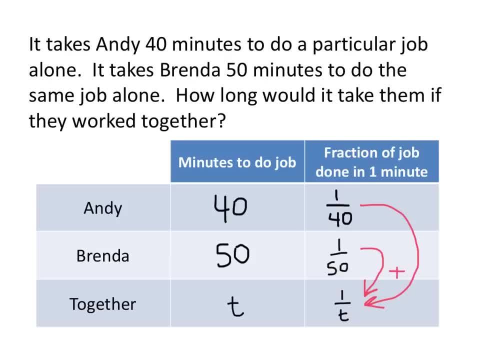 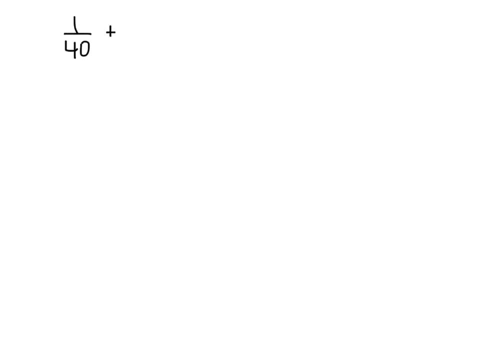 we will end up with one over t, And that gives us an equation that we can solve. Here's what that equation looks like: One fortieth plus one fiftieth equals one over t. And now let's try to see what we can do with the left-hand side there. 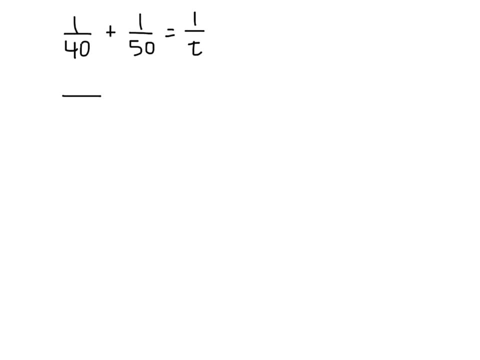 Let's find a common denominator for those two fractions. There's lots of choices, but let's use 200. It's probably the smallest that we can do. So we can get the first fraction to have a denominator of 200 by multiplying top and bottom by five. 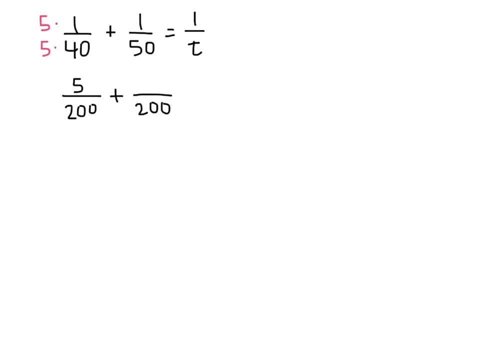 That gives us five over 200.. And for the second fraction, we can multiply top and bottom by four and we end up with four over 200. And that still equals one over t. So now we can combine the two fractions, now that they have the same denominator. 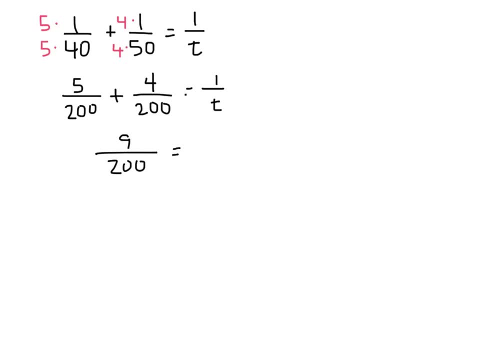 So we get nine over 200 equals one over t. We want to get the denominator of two fractions. We want to get t by itself. so we'll do a couple operations here. Let's multiply both sides by t. On the right-hand side, the t's divide out. 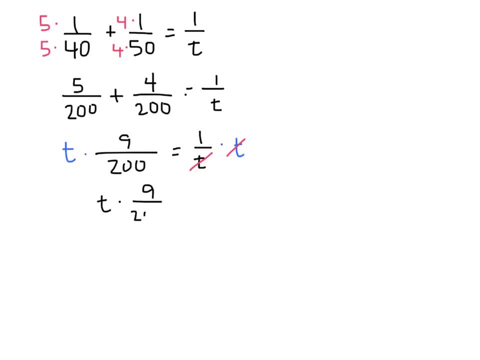 And so we get t times nine over 200 equals one. We want to get rid of the nine over 200, so let's multiply both sides by 200 over nine. On the left-hand side, the 200 and the 200 divide out. 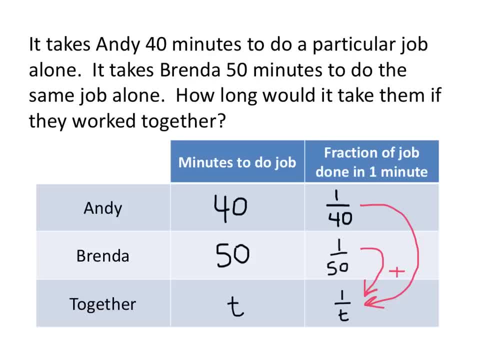 plus the amount of work that Brenda gets done in one minute. if we add those two amounts of work together, we'll get the amount of work that they get done together. So if we add one fortieth to one fiftieth, 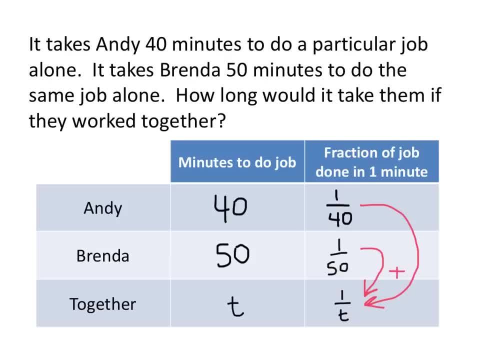 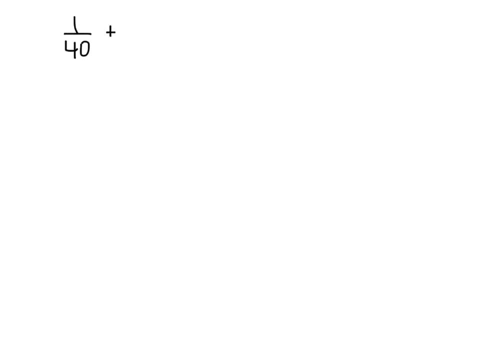 we will end up with one over t, And that gives us an equation that we can solve. Here's what that equation looks like: One fortieth plus one fiftieth equals one over t. And now let's try to see what we can do with the left-hand side there. 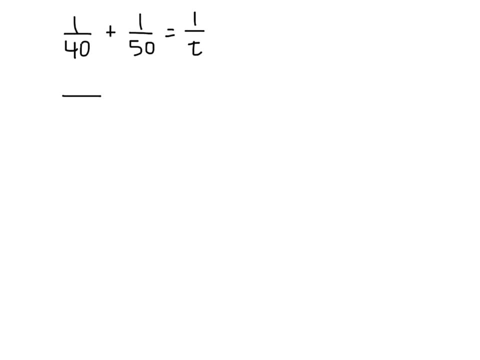 Let's find a common denominator for those two fractions. There's lots of choices, but let's use 200. It's probably the smallest that we can do. So we can get the first fraction to have a denominator of 200 by multiplying top and bottom by five. 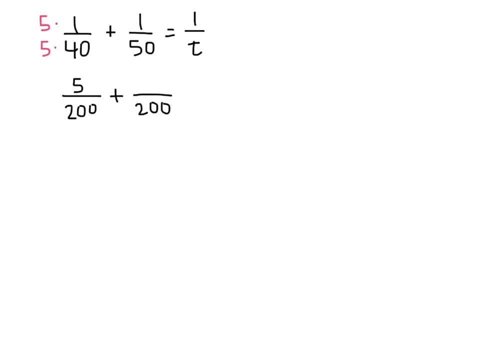 That gives us five over 200.. And for the second fraction, we can multiply top and bottom by four and we end up with four over 200. And that still equals one over t. So now we can combine the two fractions, now that they have the same denominator. 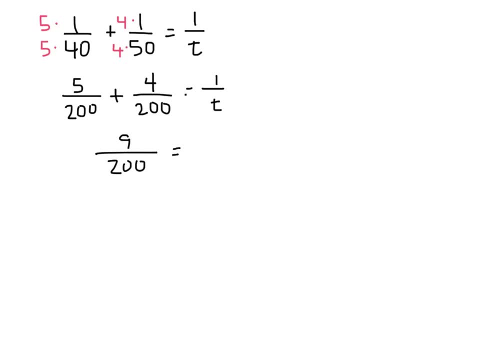 So we get nine over 200 equals one over t. We want to get the denominator of two fractions. We want to get t by itself. so we'll do a couple operations here. Let's multiply both sides by t. On the right-hand side, the t's divide out. 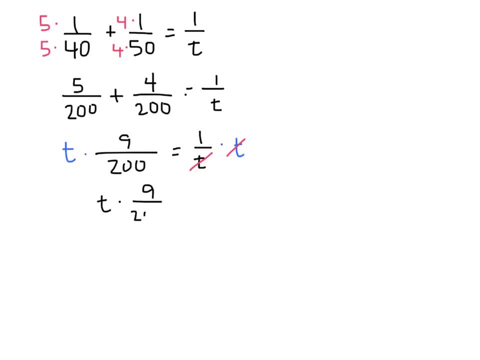 And so we get t times nine over 200 equals one. We want to get rid of the nine over 200, so let's multiply both sides by 200 over nine. On the left-hand side, the 200 and the 200 divide out. 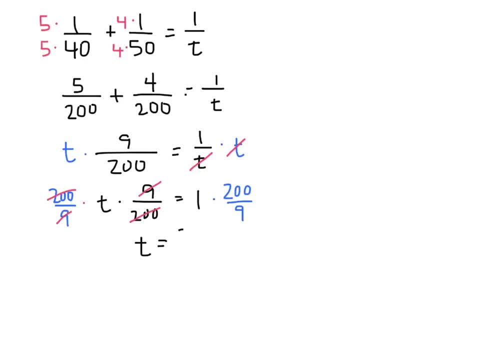 and the nine and the nine divide out, So we end up with: t equals 200 divided by nine. We can plug that into our calculator just to see if our answer seems reasonable. And we end up with 22.22, and the units here would be minutes. 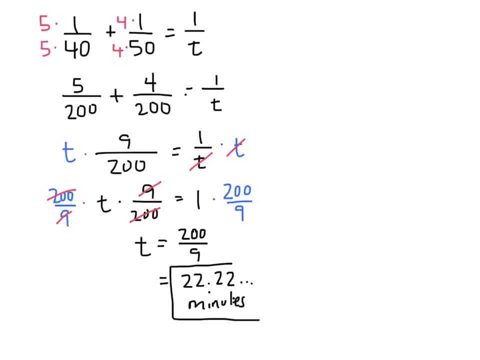 And again, that seems pretty reasonable. It took Andy 40 minutes to do it alone, Brenda 50 minutes to do it alone. So for it to take about 22 minutes for them to do it together, that seems in the ballpark And that's our answer.